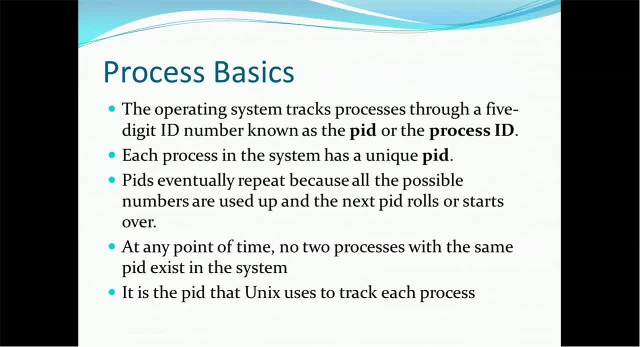 because all the possible numbers are used up and the next PID rolls or status over. It means suppose there are several processes are going on And those are completed. In that case the PID will eventually use the number which is used earlier but which is no more active. So all active processes will have the unique process ID. However, if the 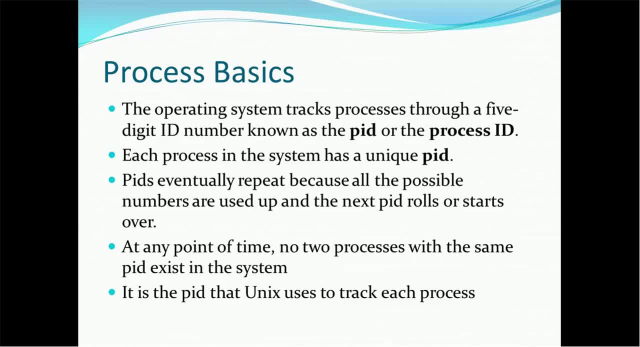 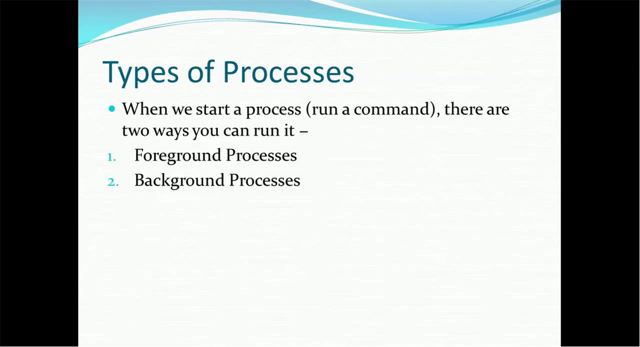 process is complete, that associated ID will be available to next process to use At any point of time. no two processes will have same PID. It is PID that Unix uses to track each process. Types of processes: Basically, there are two types of processes available. First is foreground process and 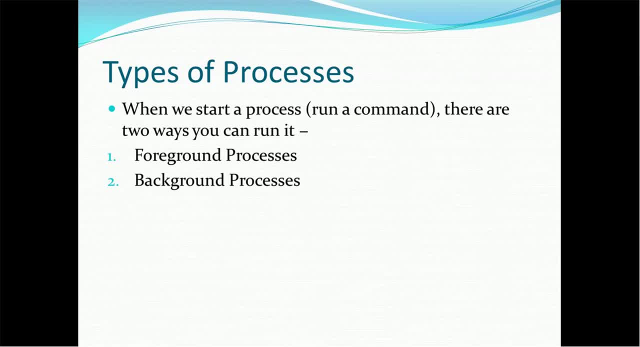 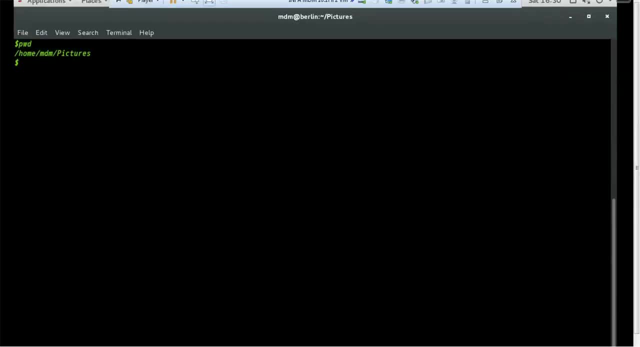 second is background process. We will see what are the foreground processes, what are the background processes. But meanwhile let's see, Uh, in Unix environment, How to identify processes. in order to identify process you have to use PS command, so it will list some. 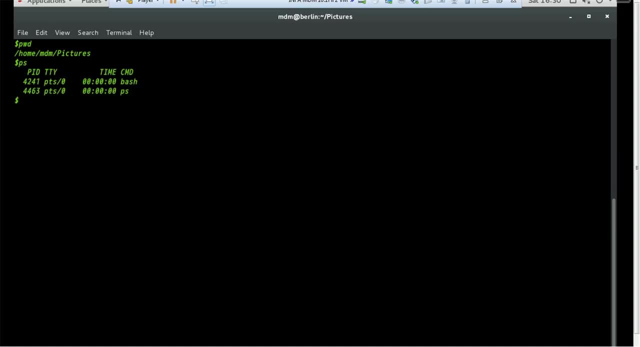 details about these processes, like PID, as we discussed, PID is a five digit unique identifier. right now it is just four digit, but it is assumed that the first digit is zero. that means this: a number is going to increase over the period of time and will limit in the five characters. so let's come back and 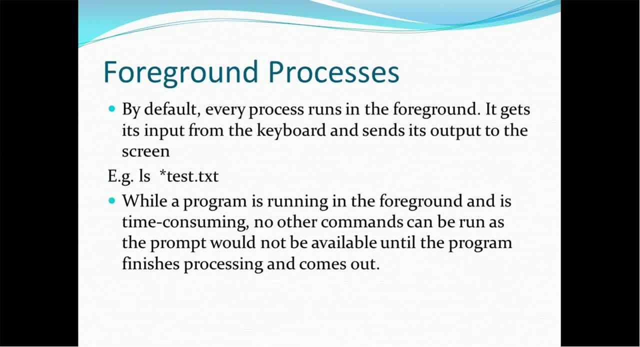 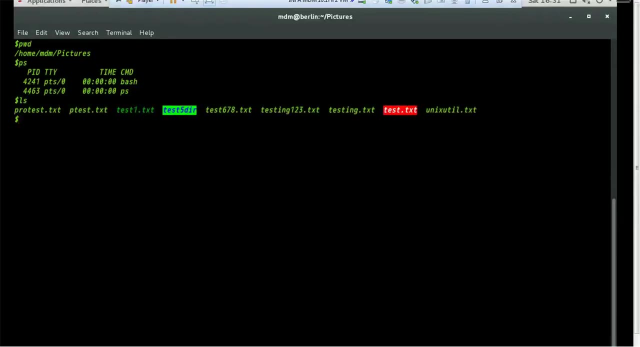 see what is foreground process or foreground processes. by default, every process runs in the foreground, so that is the default behavior of each process. it gets the input from the keyboard and sends output to the screen. for example, if you do the LS command, so that is again a process. so LS is a process. so 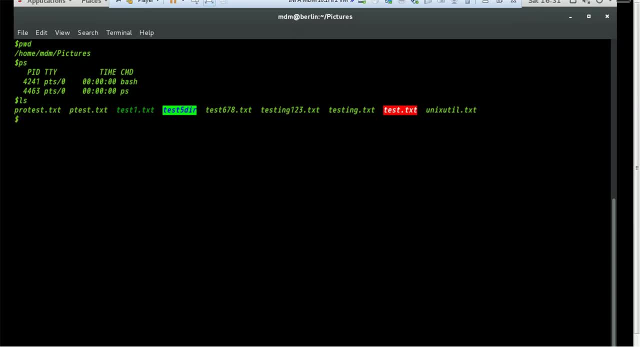 when you list the files in your given directory. it is nothing but a process for Unix. and if it print outs the output, so it takes the input. for example, if you do LS something dot txt, so the asterix dot txt is nothing but input from the keyboard. 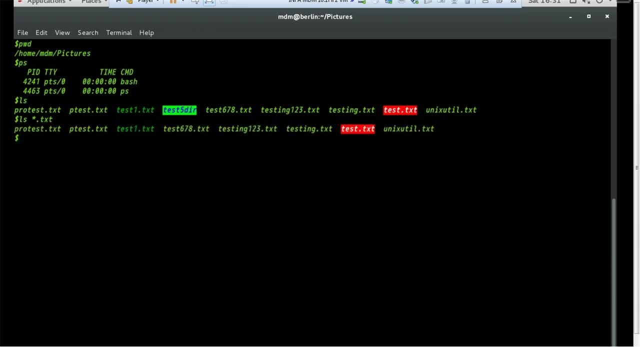 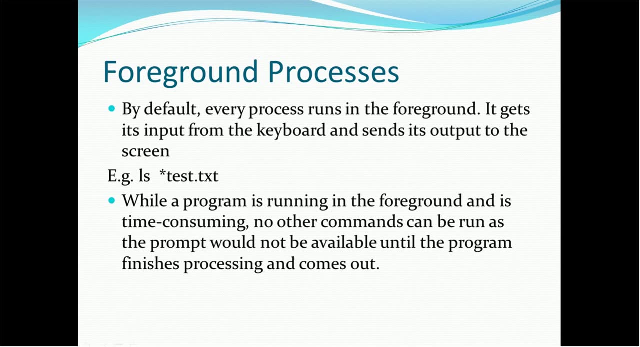 and output will be displayed in your screen. so that is the. so this LS process will be tracked as a foreground process because because it is taking the input from user and responding back to the screen while a program is running in the and it's time-consuming, no other commands can be run as as the prompt. 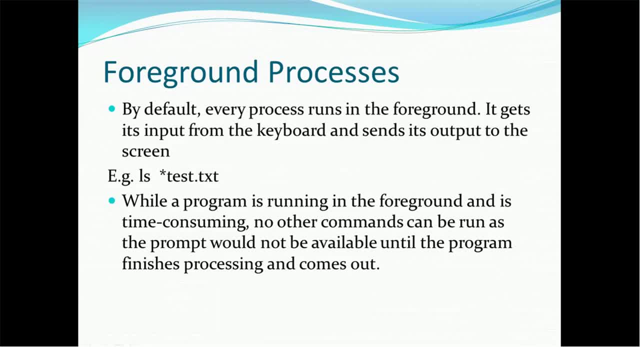 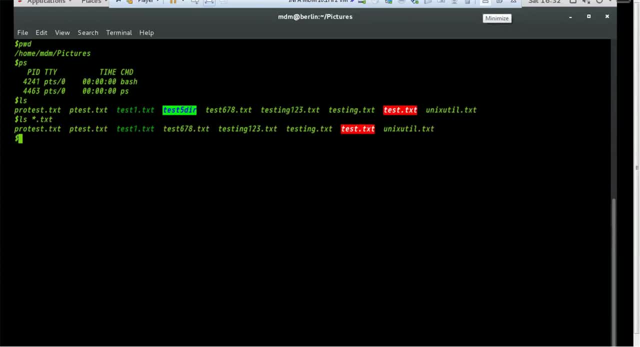 would not be available until program finishes processing and coming out. so all the most of the time the custom processes are foreground processes. so whatever we write, the process mostly accept the input and return the response. if there are long-running process, for example if I updating millions of record- 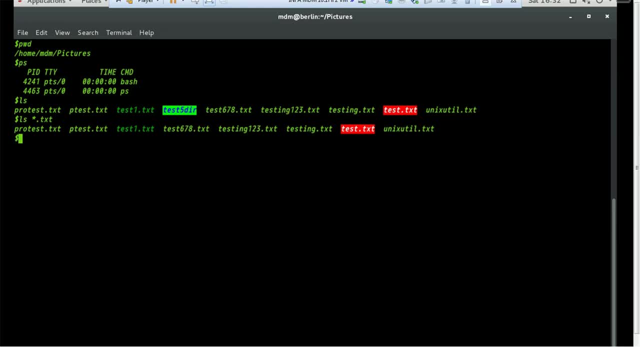 through my Unix script. so to update all the record it will take time, like maybe, suppose, few hours. so until that the command drop will not come if that process is not complete. so you will not see the next time then cursor available to execute any other process. so this kind of process is called as a foreground. 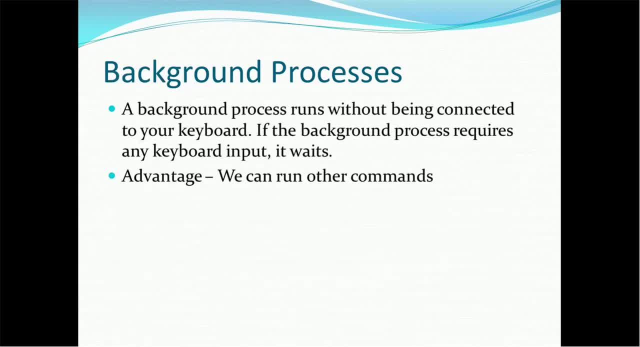 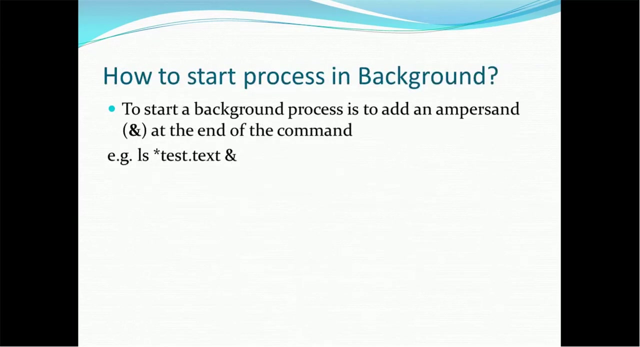 process- background process. a background process runs without being connected to your keyboard, so once you execute, the process will execute internally and the command prompt will be available to execute any other command. the big advantage of the background processes: we can run other commands because prompt will be available to use. how to start process in the background in order to 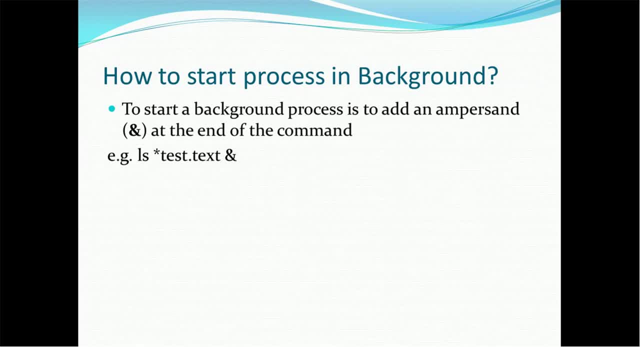 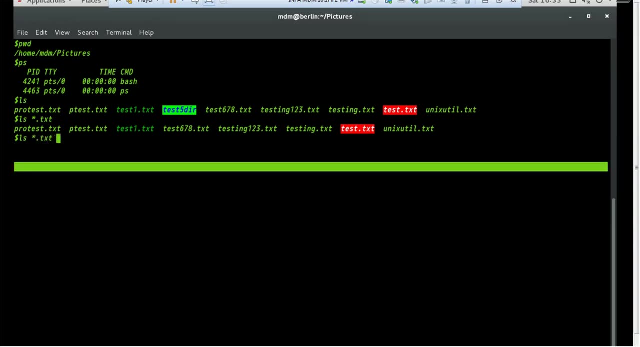 start any process in the background, you have to append and symbol at the end of command so all that process will be sent back to run as a background. for example, if you do ls and dot txt and if you use ampersand, sign or and sign, it will run this command in the background. 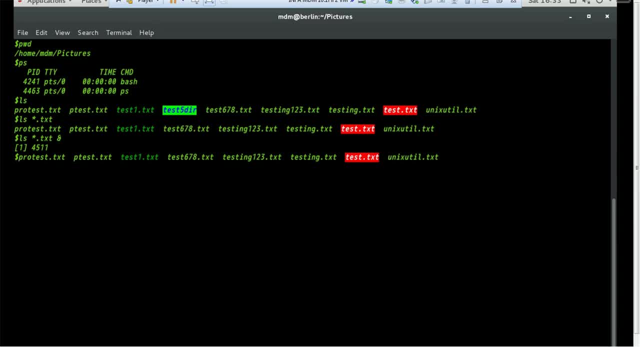 so you can see this process ID also displayed. so this process ID taking care running the process at the background once the process is complete, you can track that process also, like if you do PS, so you can see if you just enter it says this command is completed. 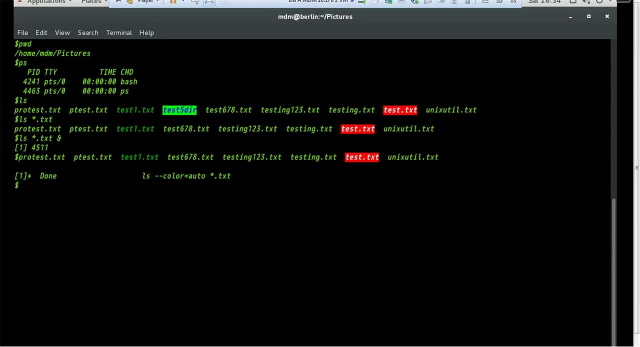 if this process is long runing, then you not see the done just status. it will be in progress, something like that. you will see, and this is process still running in the background. suppose this process is running for the long time, it is not going to kill this process. but if you just do the star dot txt and don't use 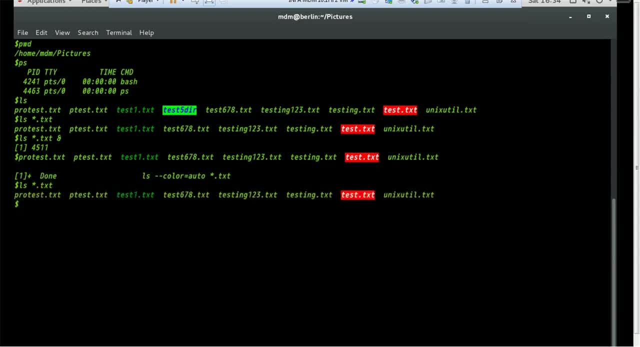 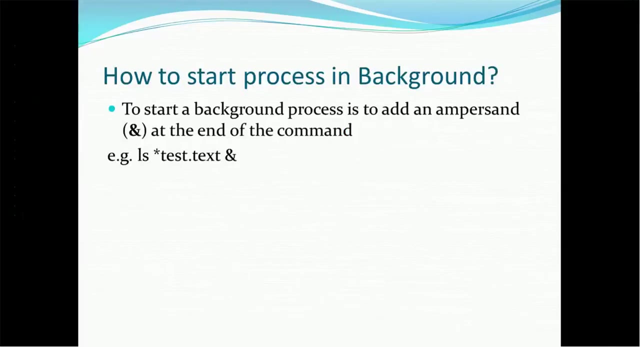 ampersand sign and enter it. County process is going continuously. if you do the ctrl c, the, you will be stopping the process. you will be killing the process so that execution will abort. so normally in real time, most of the times we use the process which get executed in the background using ampersand sign. how to? 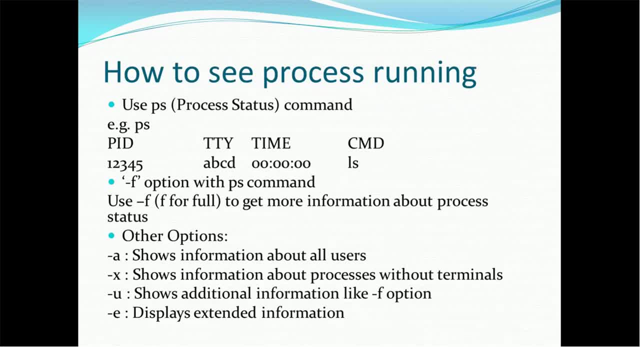 see process running. you have to run the PS command. whenever your PS command, it will give the PID, TTY, time and CMD. what these options are. of course, we can use minus app option, which will give the more details. we have the other options, such as hyphen a, hyphen X, hyphen you and hyphen e. hyphen a shows information. 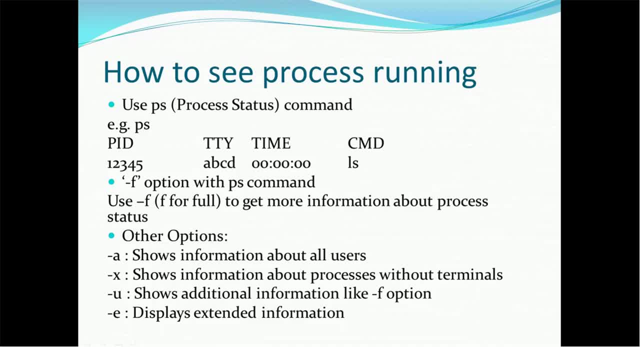 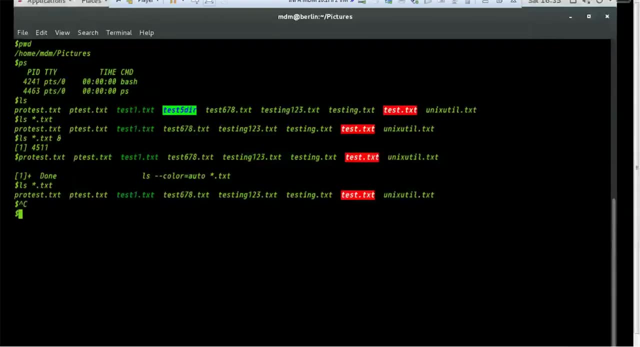 about all users. hyphen X shows information about process. without terminal hyphen. you provide additional information like hyphen a per option. hyphen e display the extended information. so to get more details let's try to use hyphen yes. for a example, if you are hyphen a, you can use user details. if you use PS minus hyphen. 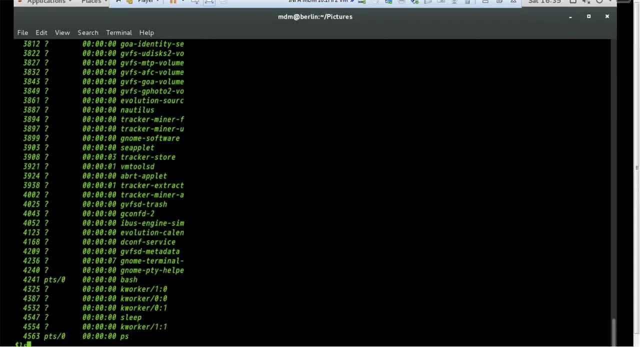 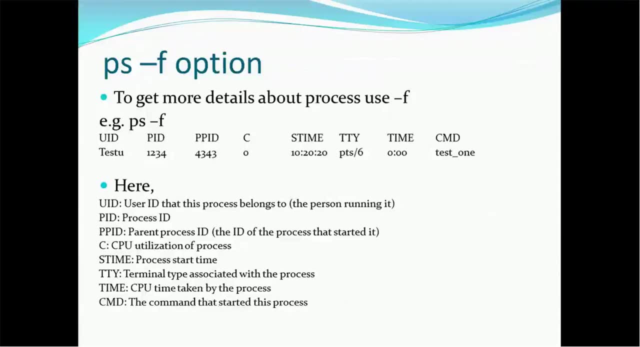 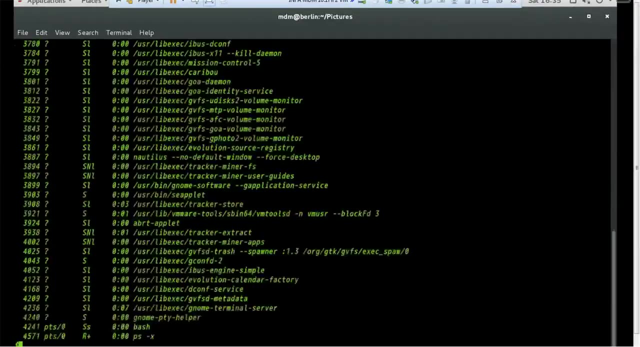 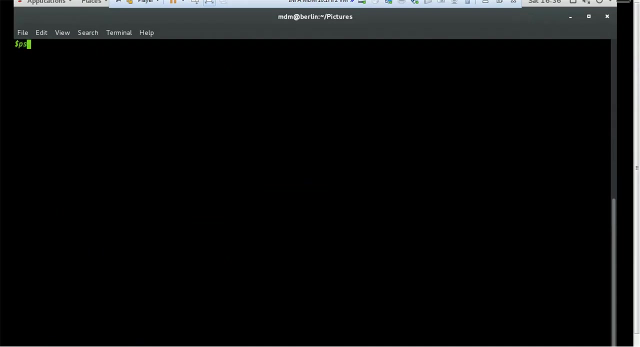 e. it will give the more details about the process. let me clear it. use PS minus. as we said, there is a for the option, like X and you. let's say what options we get. we use X. it will show the more information about the processes which are going on and PS. 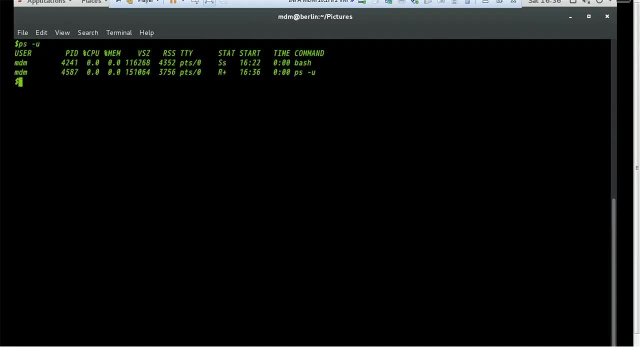 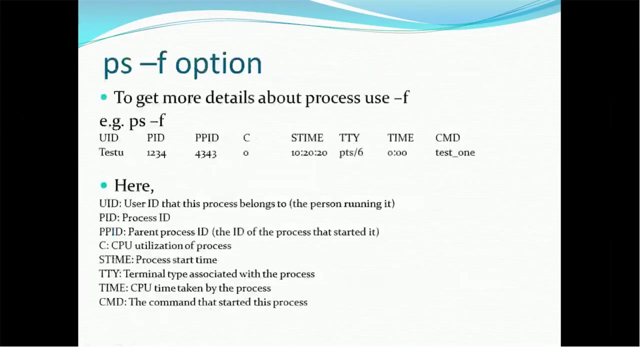 minus U. it'll. this process belongs to for a. I DS, press quit and both. this process belongs to forever. the ID is nothing but a user ID. that this process belongs to for. What is data share is what isesh 그렇죠. this is what is created. PA law is not aUID, but in the utility that data can be processed, or in expressionsca Mudra, cmd. Let's try to see what this meansItt is nothing but a. you ID is nothing but a can see that this process belongs to for other. 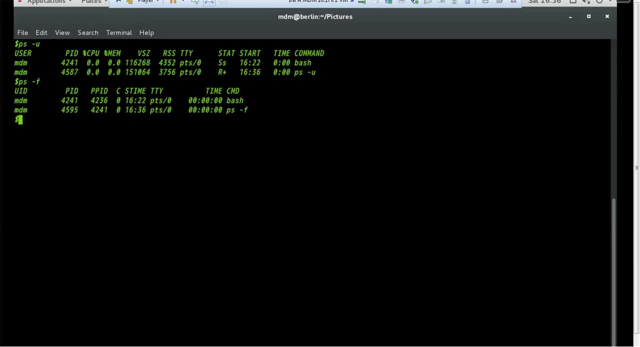 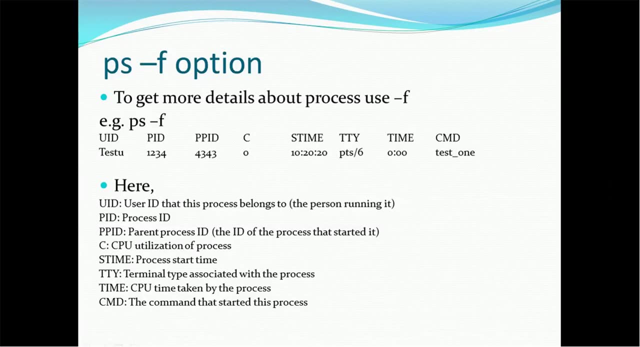 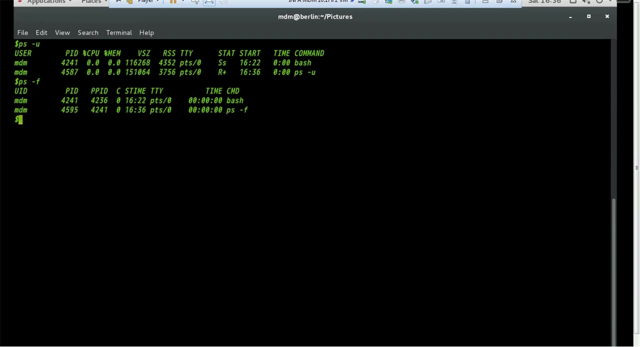 example here. MDM is the user for this bash process. MDM is user for PSF, which we ran recently. the next PID is a process ID. if you see in this process is 4, 2, 4, 1 is associated with bash command. 4, 5, 9, 5 is associated with PS. 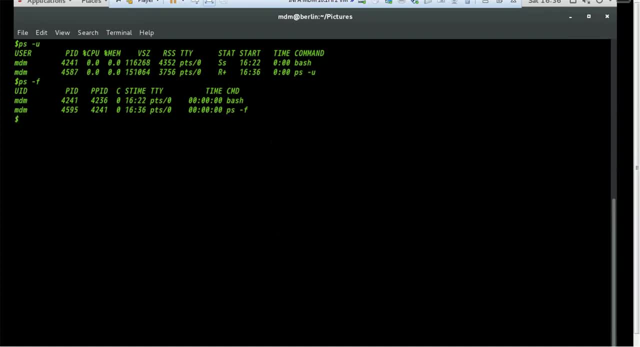 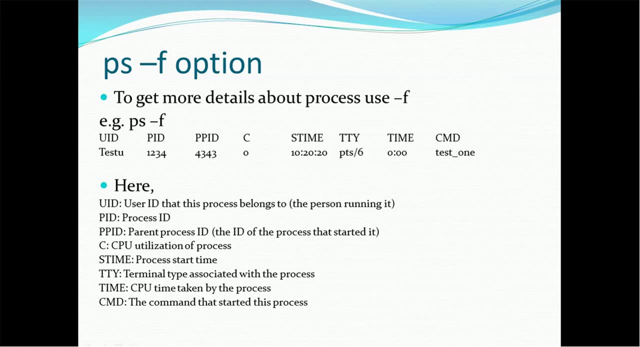 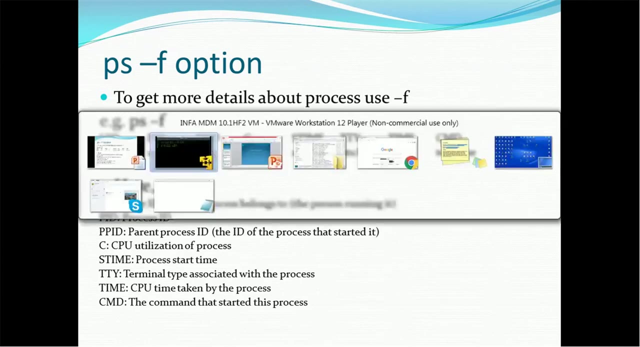 minus F command. so these are the process ID. then we have the PP ID, parent process ID. suppose there are multiple processors going on and there will be one processor as in other process. so you will see, the PID, that is PP ID, is nothing but the parent process ID which is starting this process for this bash. 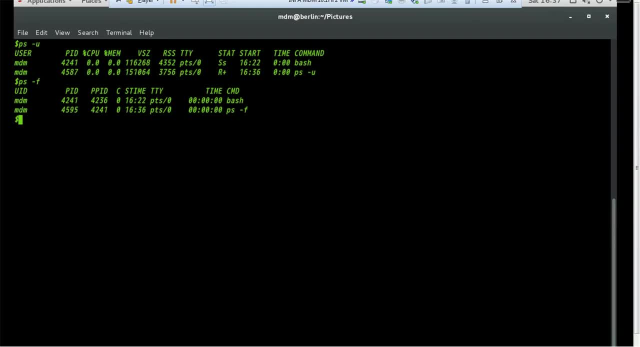 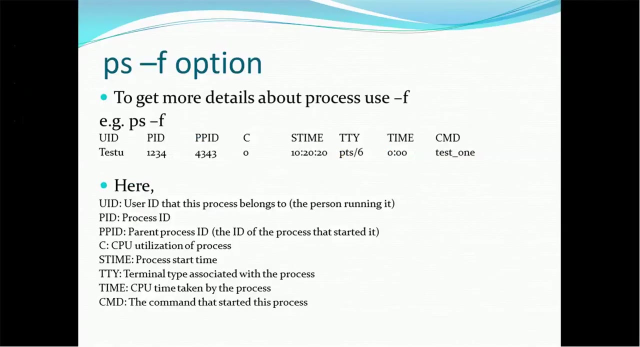 process. the parent process ID is 4 2, 3, 6. for PS minus PF. the parent process ID is 4 2, 4, 1. that means what are the bash command we are executing? its ID is the same as a parent ID because we are executing in the bash. C is CPU utilization. how much memory is? 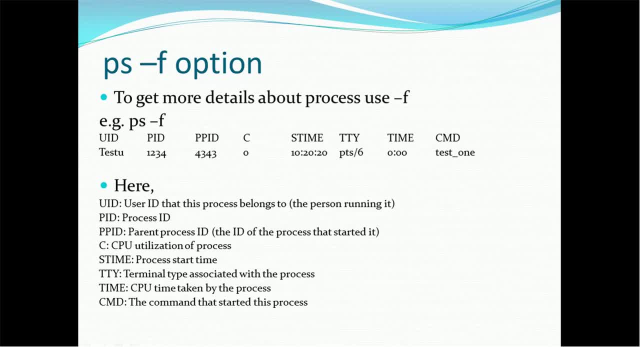 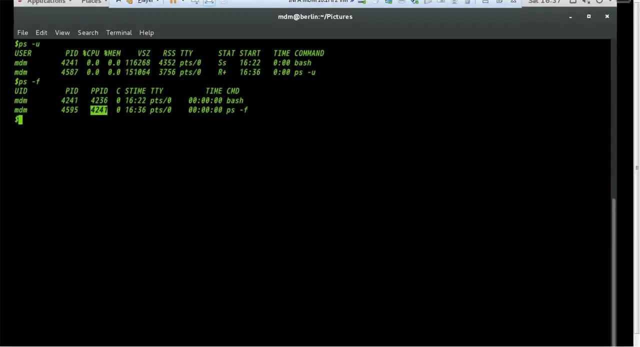 utilizing S is process time, how much time take to process TTY, the terminal type associated with the process. so let's see what are this. so you see it's CPU usage. S time is the process time. the TTY is nothing but terminal time or terminal type. then we have the time and CMD. so those are very straightforward. 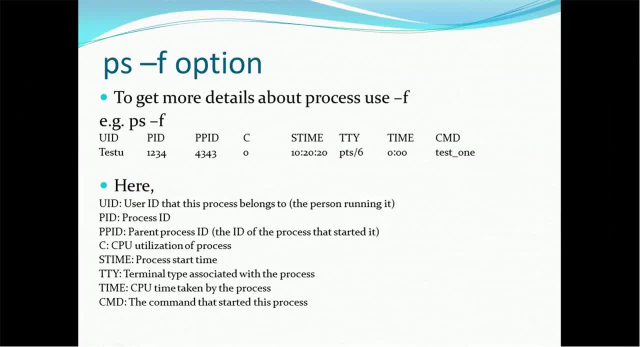 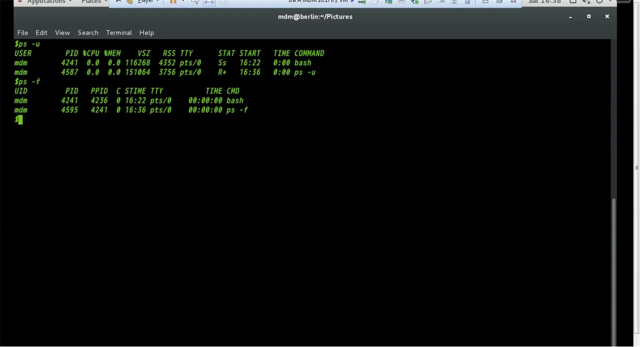 minutes time is the CPU time taken by the process and S time is like nothing, but process start time. CMD is command. what command we executed? so in this case, bash command and we have the PS minus F command, so it executed within second. that is the reason there is no millisecond shown here how to stop. 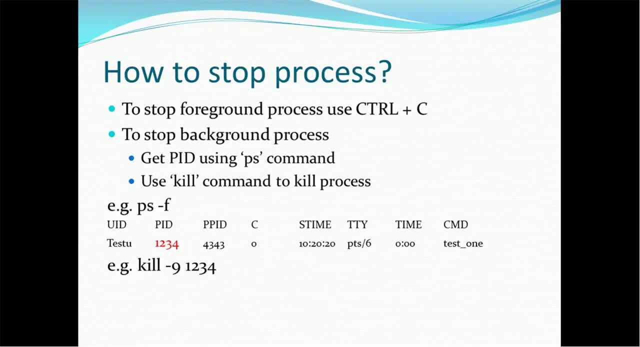 process. in order to stop process, you can for foreground process. if you use the control C, the foreground process stop immediately. if you want to stop a background process, you have to use kill command, kill minus 9 and the P ID, not parent P ID if you want to kill parent. 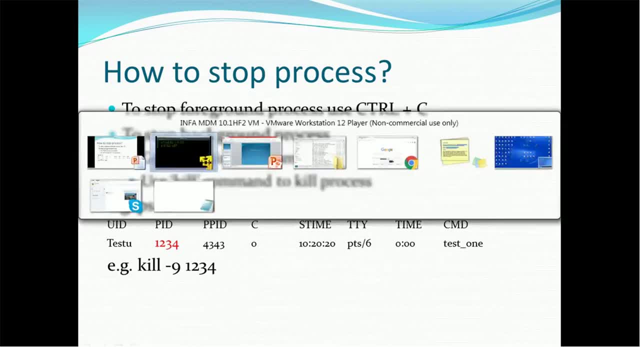 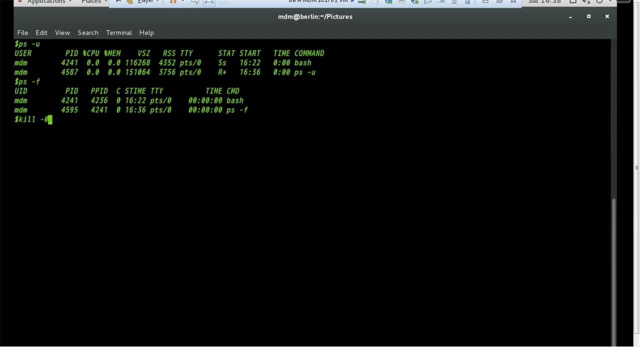 you have to kill the child and then parent. this is what recommendation. suppose you want to kill PS minus F, like you have to use kill minus 9 and you have to use process ID. for example, let me kill this four, five, nine, five, which is associated with PS minus F, so the command will look like this: four, five. 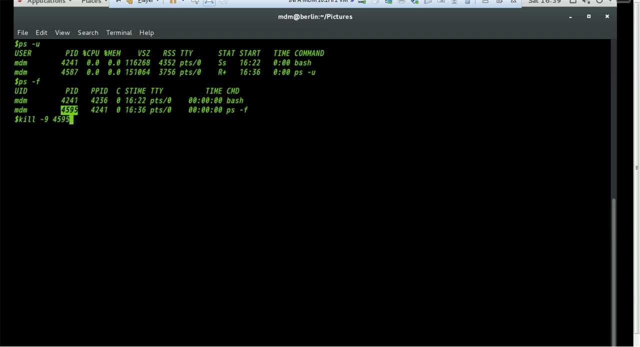 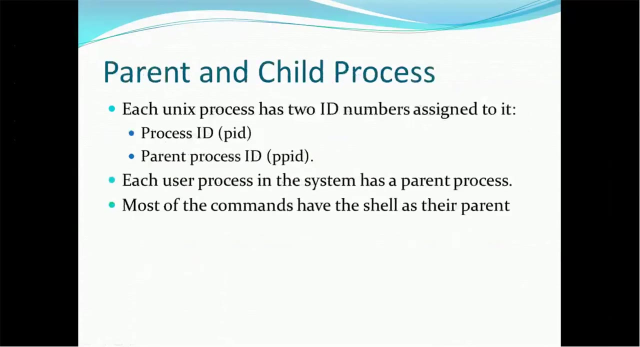 nine five. this command is already exist, stopped. let's see what it response here. so kill this command. no such process, because this process is just listing this details. so it is already completed. so there is no such process available. parent and child process. each unique process has two IDs. one is process. 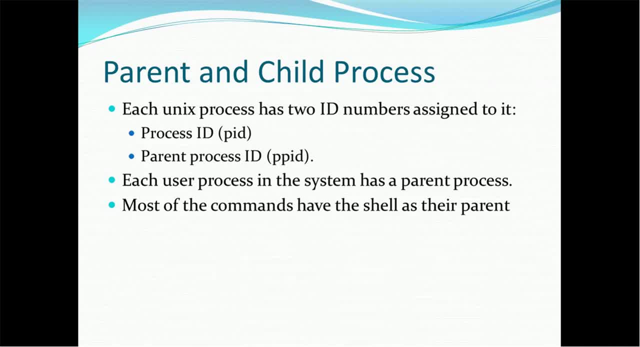 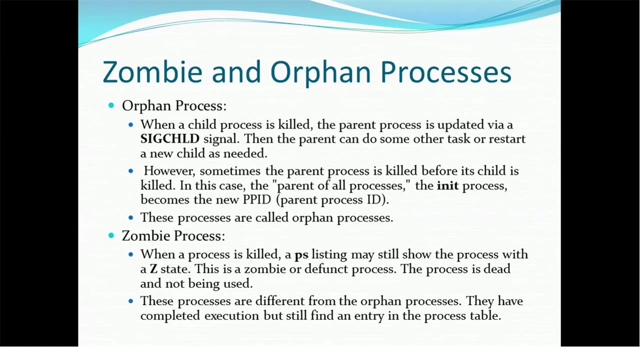 id that is pid. other is parent process id that is ppid. each user process in system has a parent process. most of the commands have the shell as their parents, like bash is our parent for commands. let's have a look on the zombie and orphan process. orphan process when a child process is killed. 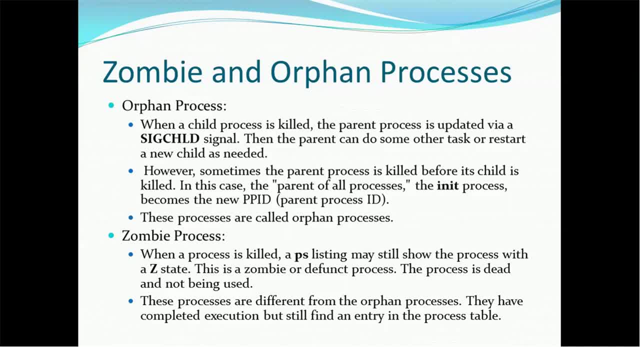 suppose if you kill the child process there will not be impact on the parent. so parent process is updated via sig, chld, that is, sick child signal. then the parent can do some other tasks or restart a new child as a needed. however, sometimes the parent process is scaled. 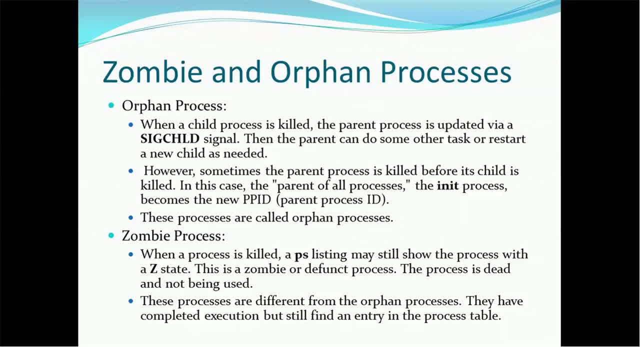 before it's a child is killed. suppose you are killing the parent without killing child. in such cases, parent of all process, the init process becomes a new ppid, that is, new parent id will be associated. these processes are called orphan processes because their parents got killed without killing child. zombie process: when a process is killed, PS. 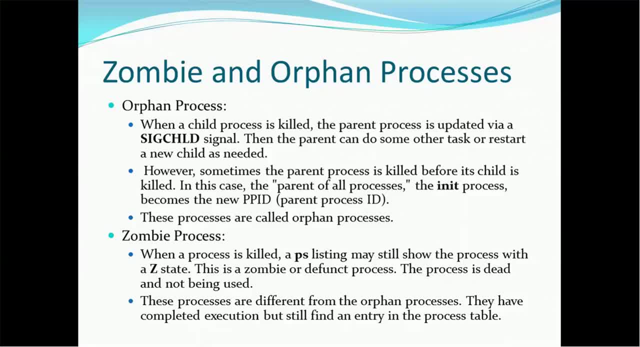 listing may still show the process with the status Z. this process are nothing but a zombie process or defunct process. the process is dead and not being used. so you will see the the process ID. but it is not a running process, it's a zombie process. these processes are different from orphan processes. orphan process are: 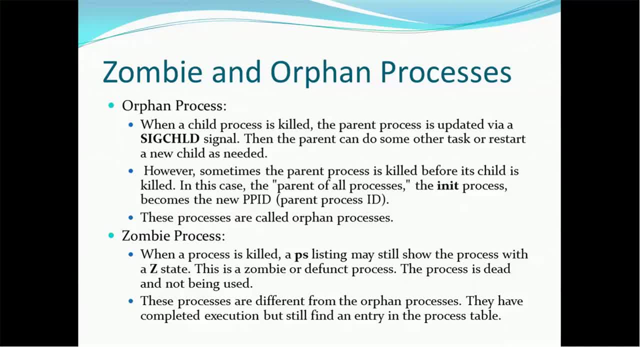 still running those, those displayed, but those are still running, but they don't have parents. however, zombie process are not running, but they still show in the memory. it's a kind of the cache a you can see in the window systems. the cache is not real data, but it is just cache information. they have the completed. 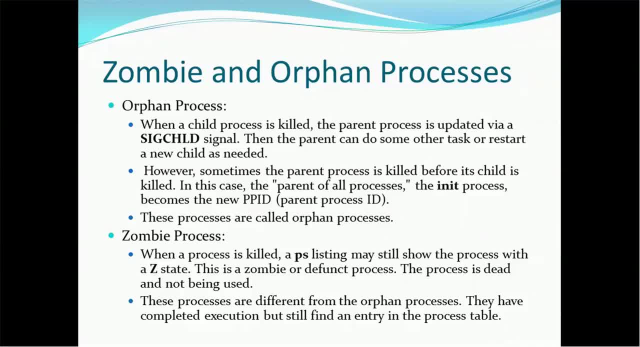 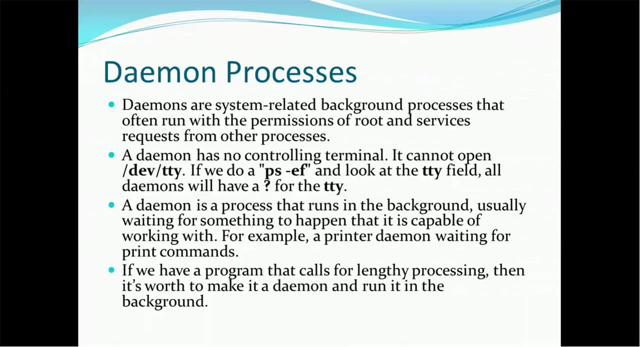 exact the the child processes completed execution but still have in okay. so zombie process, are the completed their execution but they are still showing in the process entry. there is most important processes, diamond process. so we saw there are two types of process: foreground processes and background processes. within the foreground and background processes there will be 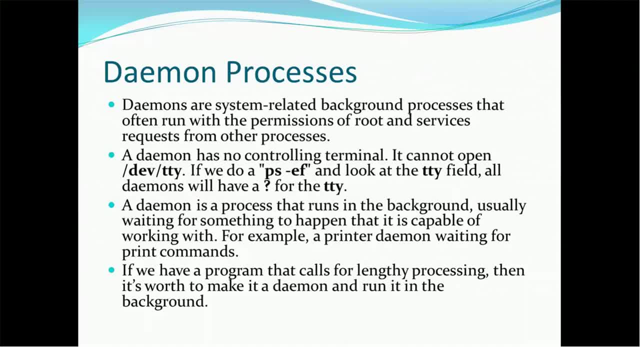 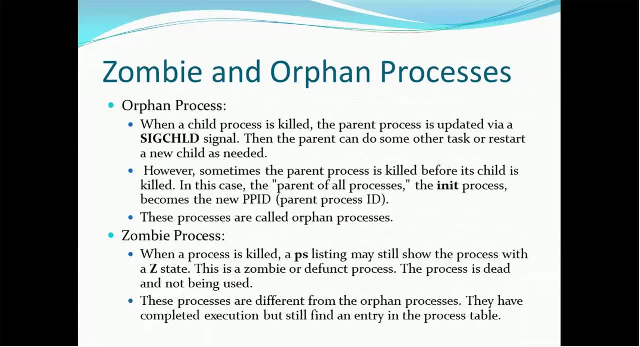 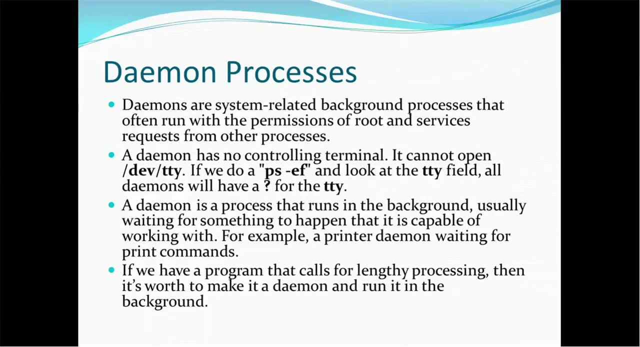 various processes like parent and child processes. there will be some processes call as the zombie and orphan processes. orphan means no parent. zombie means the process is executed, but it is have some references. the diamond process is important process. demon processes are nothing but the process is which is running behind the scene and supporting. 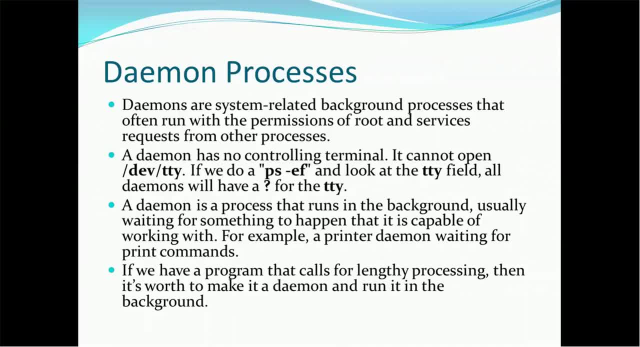 the main process. demons are the system-related background processes that often runs with the permission of the root and the services required from the, the other rig processes. a daemon has no controlling terminal. it cannot open dev tty. that is terminal. if we do a ps minus ef and look at tty field, all daemon will have a question for the tty. so let's 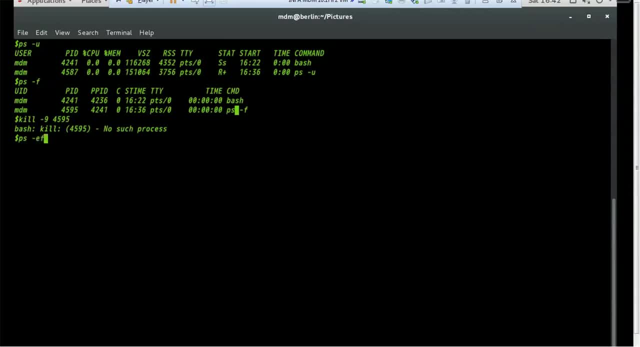 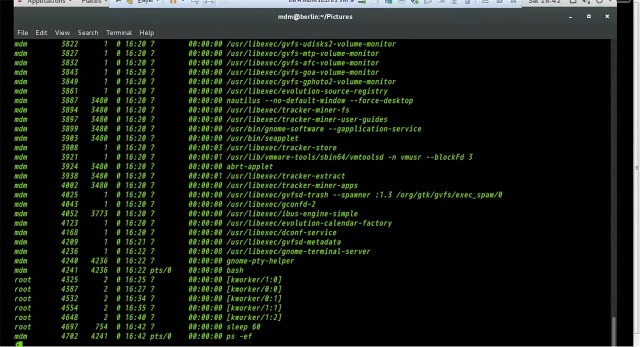 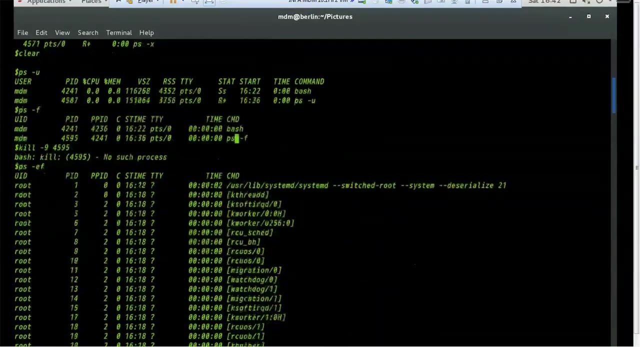 try out that. if you do the ps minus here, so if you see the question mark, so tty, if you notice there is no terminal associated with this, let me show you that from top. if you see tty, it is question mark, no terminal associated. so this process is a daemon process. so all these processes, 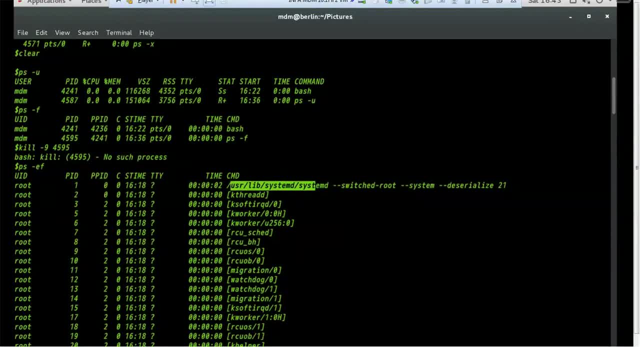 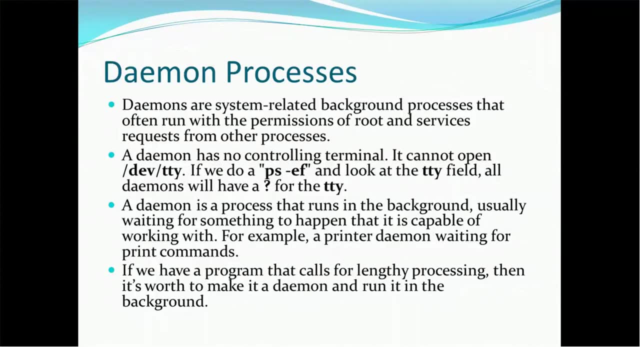 with question mark are listed are nothing but the daemon processes. a daemon is a process that runs in the background, usually waiting for something to happen. that is waiting for something to happen, capable of working with, for example, printing daemon, waiting for print commands. so printing daemon is continuously running. even we can't see as a ps command. if you do the ps minus ef, it will. 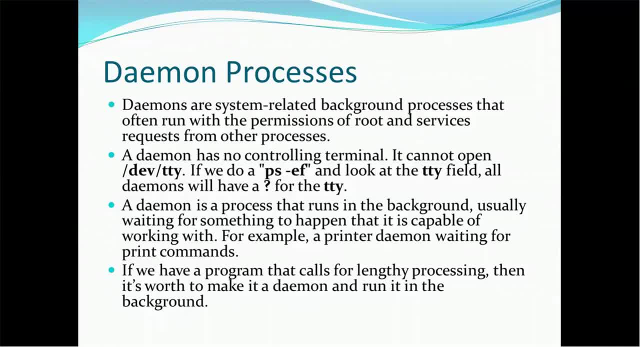 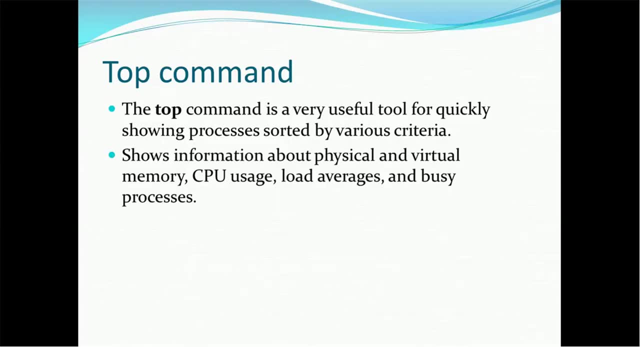 show us. if you have a program that calls for lengthy processing, then it was to make it as a daemon and run it in the background top command. the top command is very useful, very commonly used by people who have a lot of experience in working with other programs, so it's very useful that you 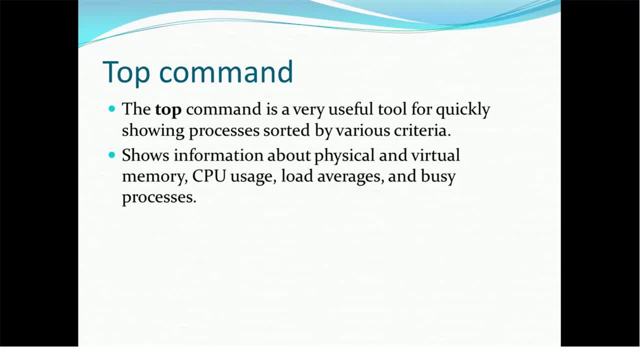 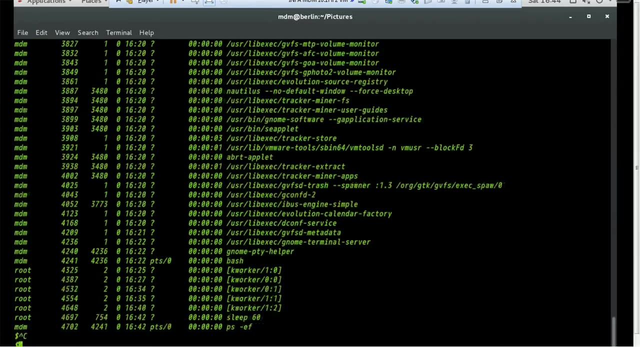 can run this organically and do work on it. now here we have a tool called top command. this is an Municipal Process Unit called top command which can do the task of doing a brief operation of a computer to run the process simply by clicking on the top command and it will perform. 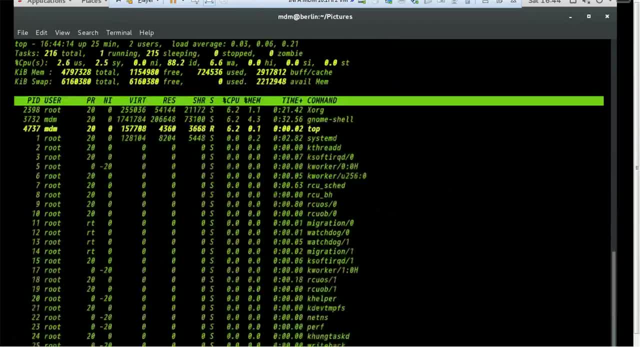 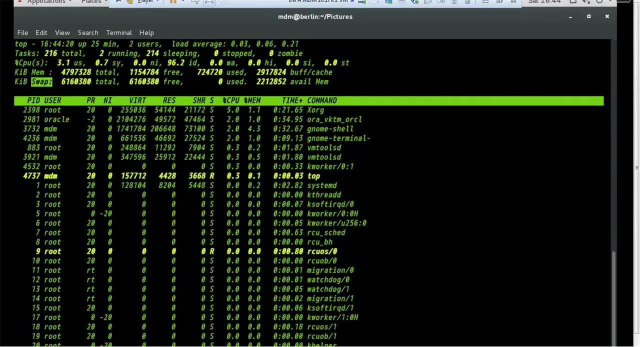 it will run the entire process, so let's see what it can do. so this is where it's going to run the process, so it will run that. if you run it on the top command, let me show you how to do this. or assign what is the swap memory? total memory, free memory: how much free memory are available? 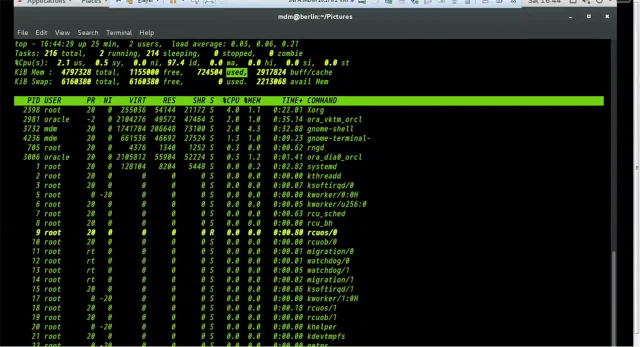 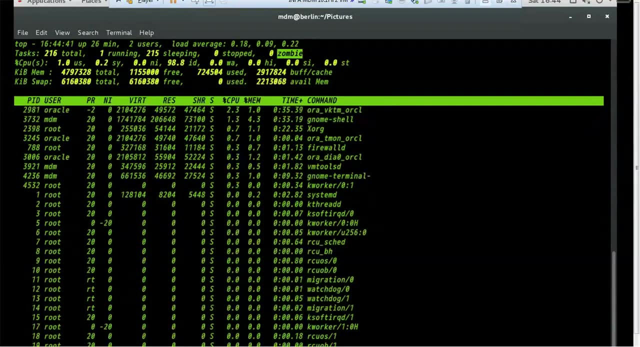 use memory, etc. so all these memories mentioned here, how many processes are running, how many processes are slipping, how many processes stop, how many zombies are there? so, looking at this zombie, you can able to control and you can stop those. so by that way, you can release those processes. 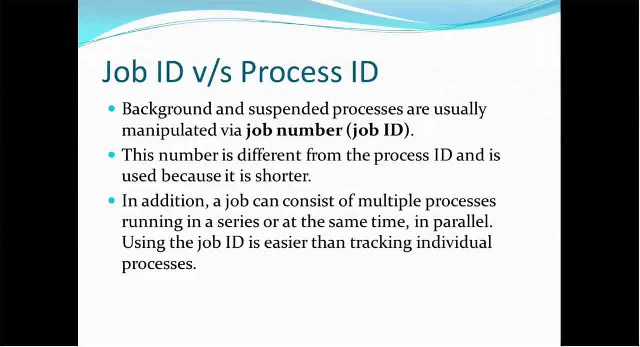 or you can kill those processes. job id versus process id, background and suspended process are usually manipulated via job id, so background and suspended processes keep remember this. this number is different from the process id and usually and used because it is shorter. in addition, a job can consist of multiple processes running in a series or at a same time in parallel. 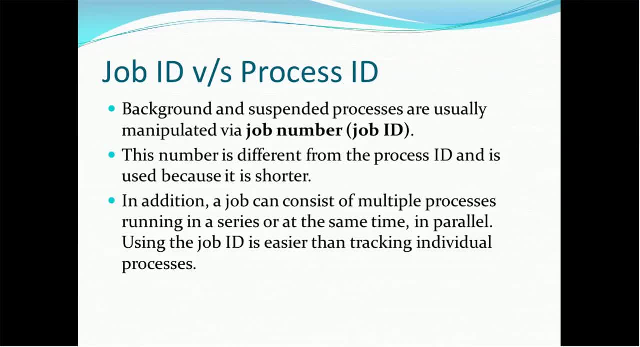 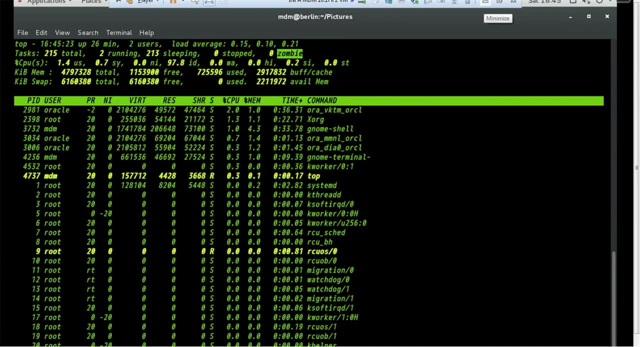 using the job id is easier than tracking individual process. that is, these are the differences we have. i hope this short tutorial give you idea how to handle the processes, how to determine the processes, what are the zombie process, what are the daemon process, etc. um, if you have any questions or queries about unix tutorial, you can definitely. 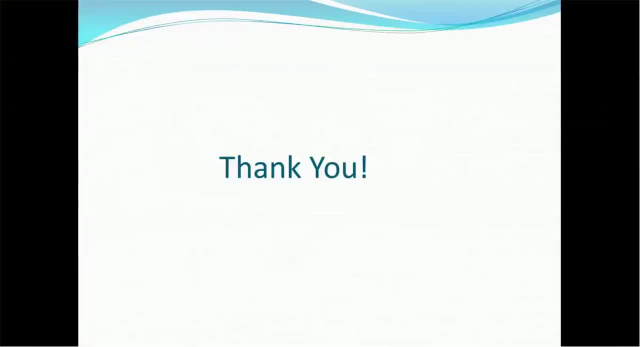 mention the comment section of this video. thank you again and have a nice time.